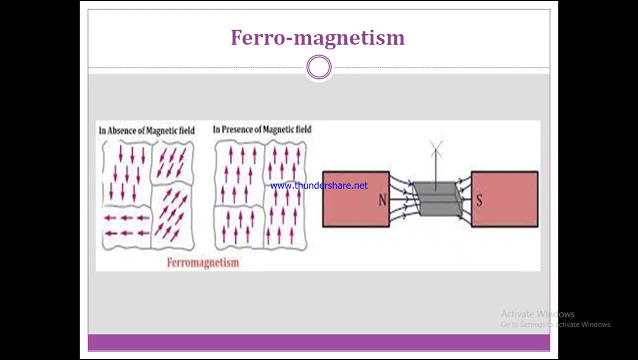 So the ferromagnetic material have a strong interatomic interaction, due to which they exhibit an ordered magnetism Means. if the ferromagnetism material is placed in a magnetic field, then the dispersed magnetic dipoles are converted into a magnetic field. 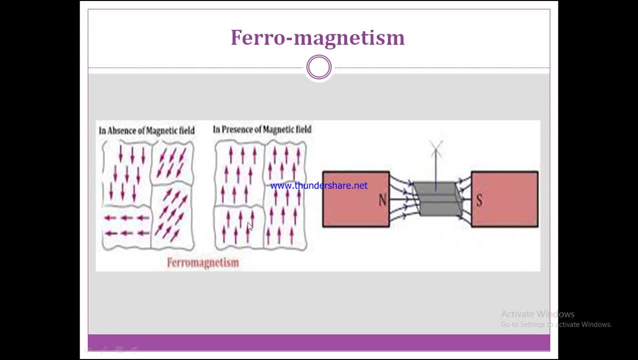 This is the parallel structure of magnetic moments. According to that, the magnetic flux lines flowing from N to S are structured in parallel manner. As we know, in the absence of a magnetic field, the ferromagnetism behaves in dispersed magnetic dipoles. 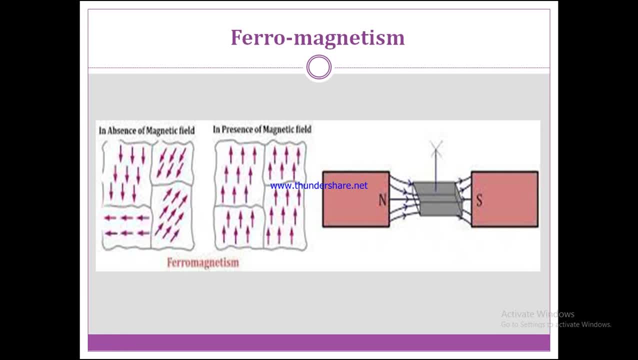 In a disordered manner, But when it comes in the presence of a magnetic field, then the magnetic dipole moments structure is converted into a parallel structure Or it becomes in the parallel position. Now both the paramagnetic and diamagnetic material are connected in parallel. 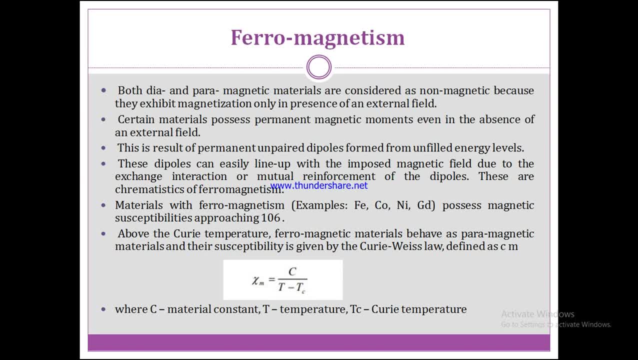 Now both the paramagnetic and diamagnetic materials are considered as non-magnetic, because they exhibit magnetization only in the presence of an external field, In that certain materials possesses permanent magnetic moments even in the absence of an external field, which results of permanent unpaired dipoles formed from unfilled energy layers. 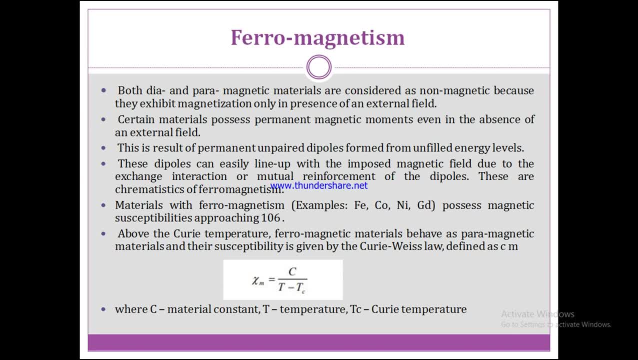 Now these dipoles can easily line up with the imposed magnetic field And due to that, the exchange, interaction of mutual reinforcement of the dipoles. These are characteristics of the ferromagnetism material. Now the materials with ferromagnetism should be consistent. 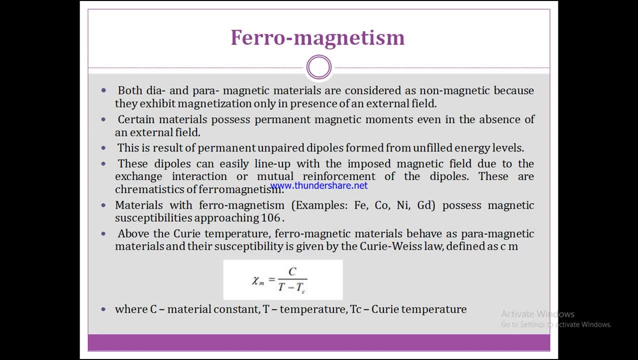 Now the materials with ferromagnetism should be consistent. The first, of ferrous, copper, cadmium and neon, possesses the magnetic susceptibilities approaching 10 raise to minus 6.. The first, of ferrous, copper, cadmium and neon, possesses the magnetic susceptibilities approaching 10 raise to minus 6.. 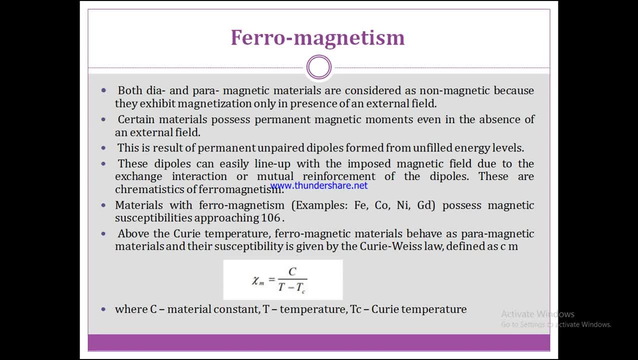 In above the Curie temperature. Ferromagnetic materials behave as paramagnetic material and their susceptibility is given by the Curie-Weiss law, which defines: as XM is equal to C upon P minus PC, where the C is nothing but the material constant, the capital T is nothing but the temperature and PC is nothing but. 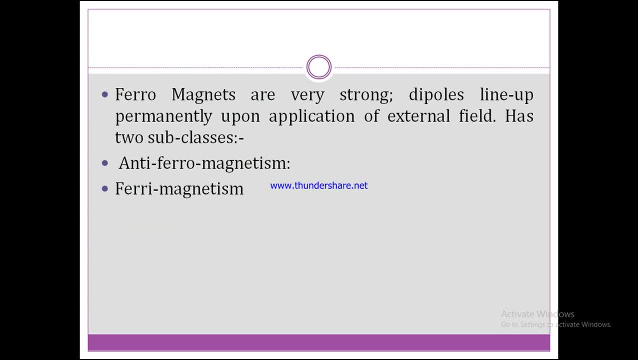 the Q-radian pressure. now, the ferromagnets are very strong in a nature. their dipoles are lines up permanently upon the application of external field and has the two subclasses which are known as anti-ferromagnetism and ferromagnetism. 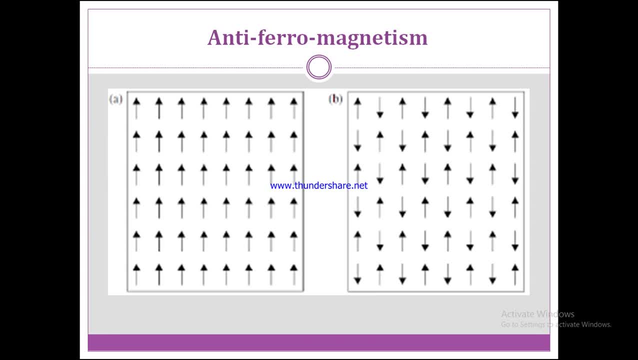 now this is the structure of anti-ferromagnetism as shown in the figure. if the neighboring dipole moments are aligned in anti parallel, then the material is known as antiferromagnetism Australia and this phenomenon of magnetic dipole movement getting aligned anti the 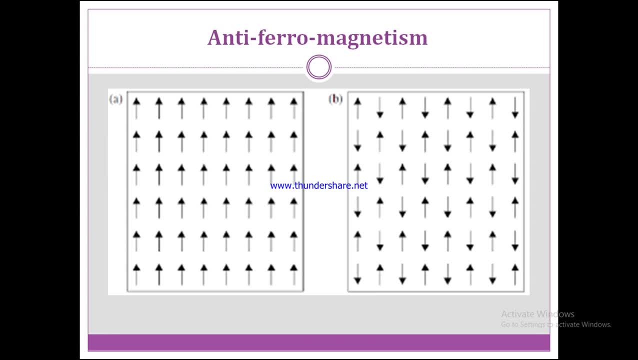 matter knew the anti-ferromagnetism In this structure. the figure A- should be called should be- shows the ferromagnetic material, whereas the figure B it shows the anti-ferromagnetic material structure. In the ferromagnetic material a large resultant magnetism is observed. 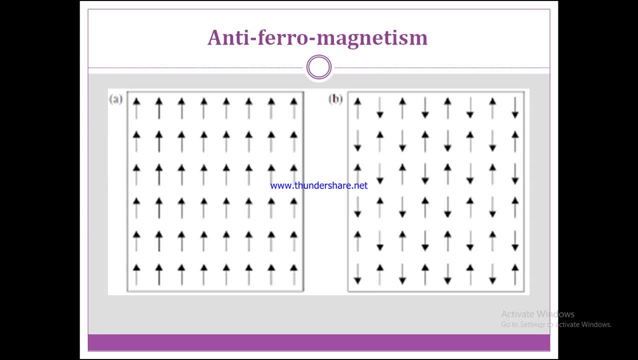 but in anti-ferromagnetic material the resultant magnetism is zero. In the ferromagnetic material, if there are four atoms per molecule, then the molecular moment will be four times the atomic moment. But in anti-ferromagnetic material the molecular moment will be four times the atomic moment. 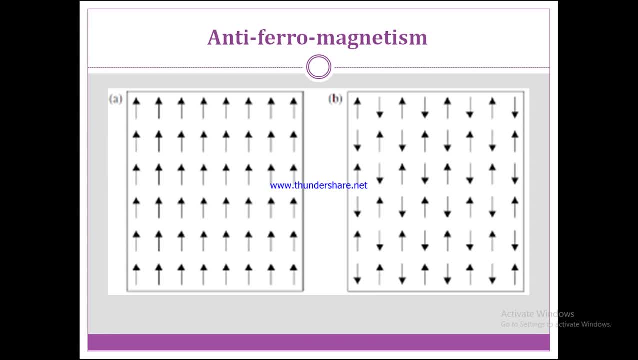 But in anti-ferromagnetic material the molecular moment will be zero and therefore the spontaneous magnetism will be absent. Now in a figure B, you just observe that the magnetic dipole moments which are placed between the particular structure, 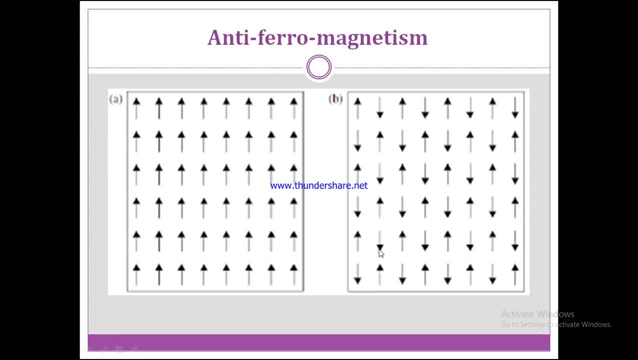 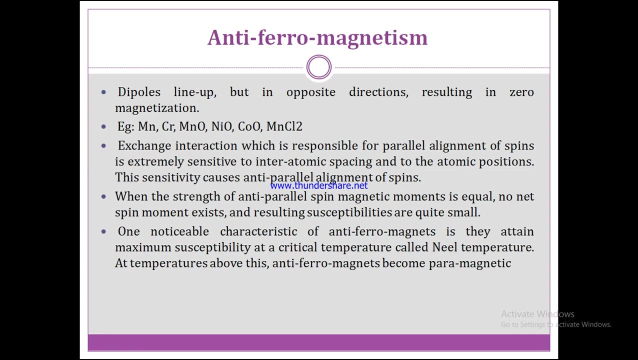 it will be having the opposite direction to each other, And because of that it should be called as the anti-ferromagnetism or anti-ferromagnetic materials with each other. Now, in this type of material, the dipoles are lined up, but in opposite directions. 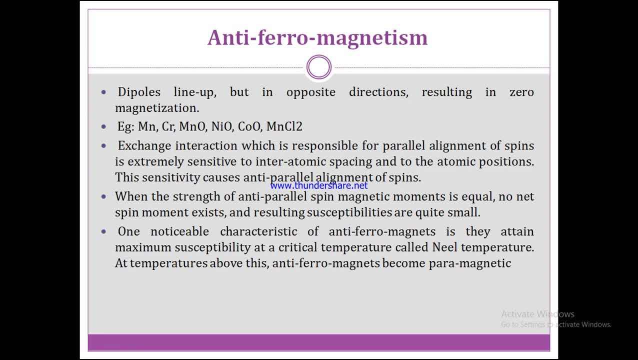 resulting in a zero magnetism. The examples for anti-ferromagnetism materials are the magnesium chromium, that is a thing called CR, MnO, NiO, COO, MnCl2.. Now if we exchange the interaction which is responsible for parallel alignment of a spin, 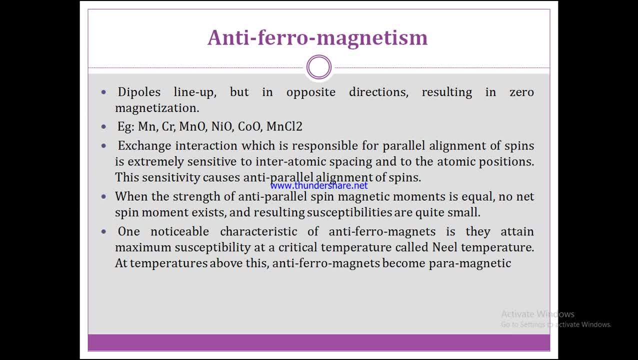 it is extremely sensitive to inter-atomic spacing and to the atomic position. This sensitivity causes anti-parallel alignment of a spin. When the parallel alignment of particular structure of a dipole moment is to be there, then the alignment of spins is extremely sensitive. 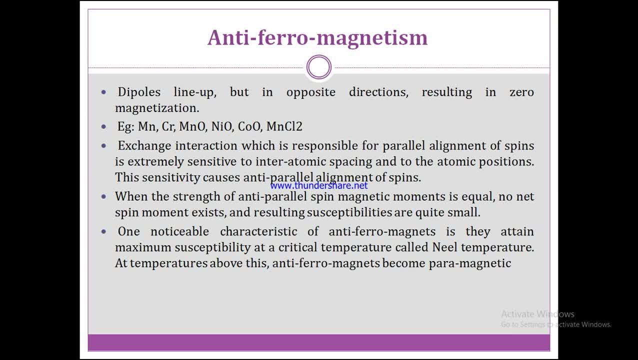 When the parallel alignment of a dipole moment is to be there, then the alignment of spins is extremely sensitive to the inter-atomic structure, that is to say the spacing between the two orbits, And due to that the atomic positions of an atom should be having the higher sensitivity. 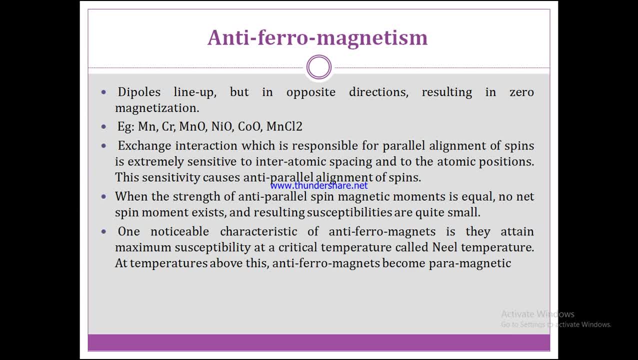 which causes the anti-parallel alignment of a spin. When the strength of anti-parallel spin increases, the anti-parallel spin magnetic moment is equal. no net spin moment exists and the resulting susceptibilities are quite small. When the strength of anti-parallel spin of magnetic moment, 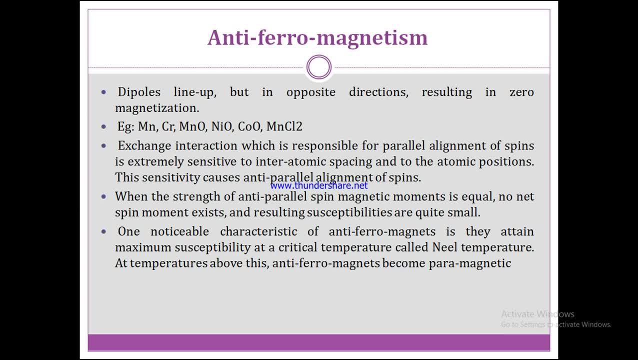 which is equal having no net spin moment exists, and therefore these resulting susceptibilities are quite small. One noticeable characteristic of anti-parallel magnetic material is that they attain maximum susceptibility at a critical temperature called nil temperature, And at temperatures above these its anti-parallel magnets becomes an paramagnet. 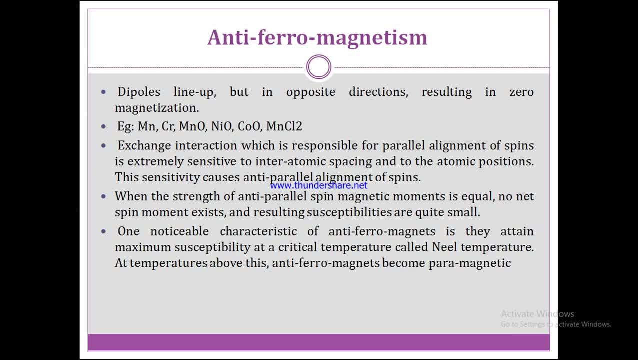 Hence what the magnetic material properties, which should be depends upon the temperature, is showing that when the anti-parallel magnetic material is having the maximum susceptibility up to the critical temperature only, which is called as a nil temperature, And above that particular temperature, 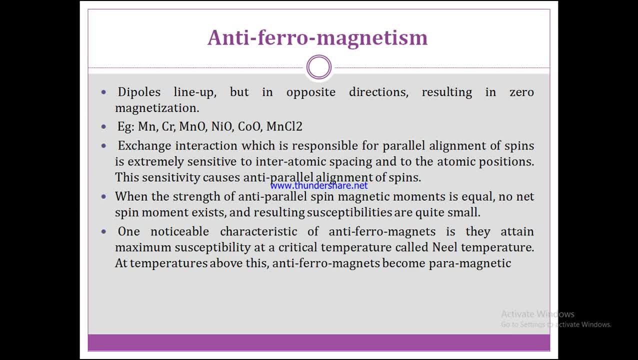 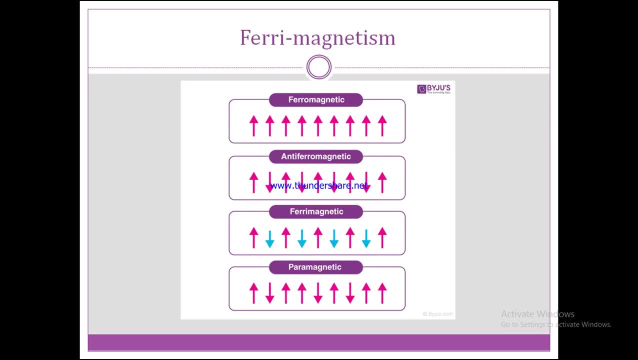 the anti-parallel magnetic material should be, converts its behavior to the paramagnetic material. The next one is nothing but the ferrimagnetic material. If the order of the magnetic moments is shown in figure number 3,, that is nothing but the ferrimagnetic material. 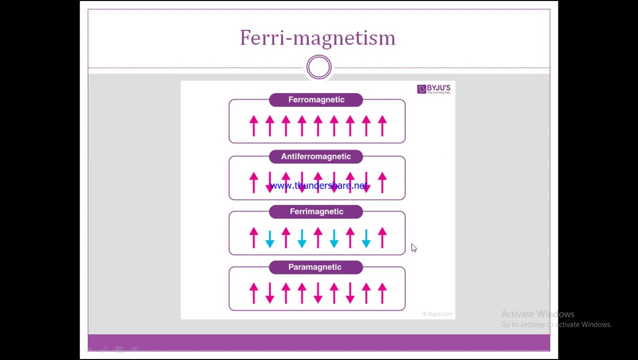 the material is known as the ferrimagnetic. In this the value of molecular moment of ferrimagnetic material is in between that of the anti-ferromagnetic material and ferromagnetic material. The arrangement of magnetic dipole moments of the ferrimagnetic material. 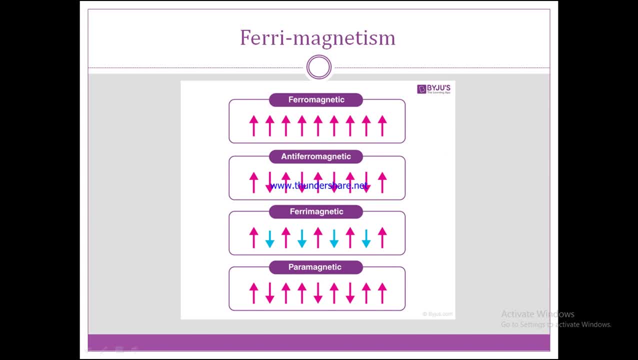 is shown in the figure. Now, as we know, we have discussed about the ferromagnetic, anti-ferromagnetic and paramagnetic material. The ferrimagnetic material is having the magnetic dipole moment direction same as that of anti-ferromagnetic material. 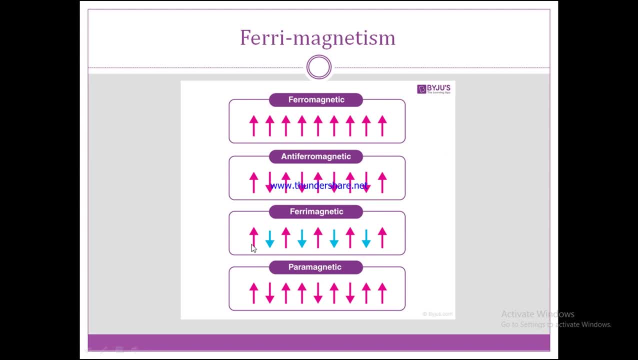 that should be nothing but the opposite to each other. But the difference is that in anti-ferromagnetic material the presence of such dipole moment are near to each other which are having the opposite spin of that particular molecule. But in ferrimagnetic material, 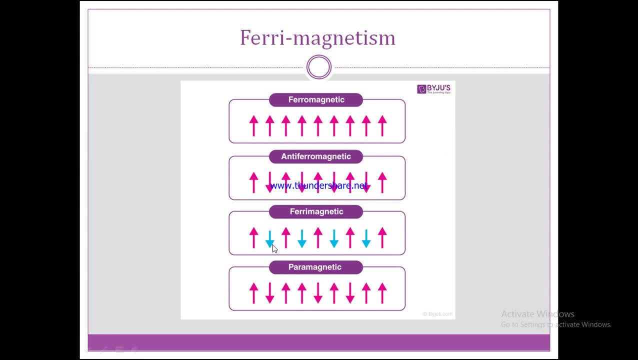 the resultant opposition of the magnetic dipole moment should be having the different types of magnetic material which should be available in ferrimagnetic material. Now, as we discussed the four types of magnetic materials over here, we will revise some parts regarding that one. 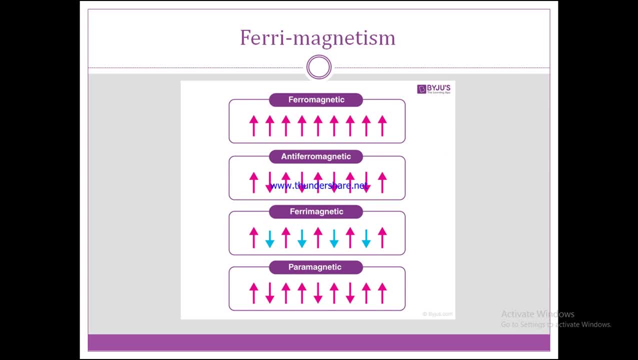 In a diamagnetic material- we have studied that or discussed that- the permanent dipoles are absent. the arrangement of that dipole moments are not applicable and the interaction between the neighboring dipole is also not applicable In a paramagnetic material. 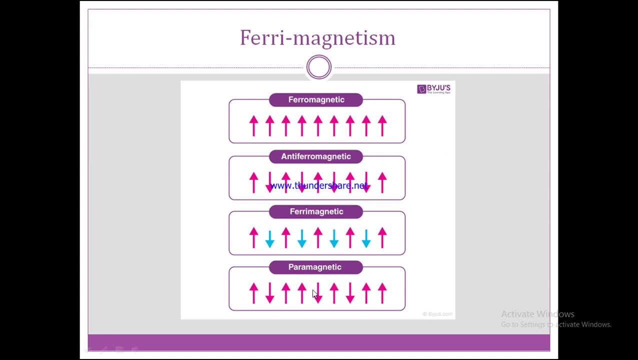 the permanent magnetic dipoles are present. the structure of that paramagnetic material is shown in this figure and the interaction between the neighboring dipoles is zero or negligible. In a ferromagnetic material, the permanent dipole moments are present. 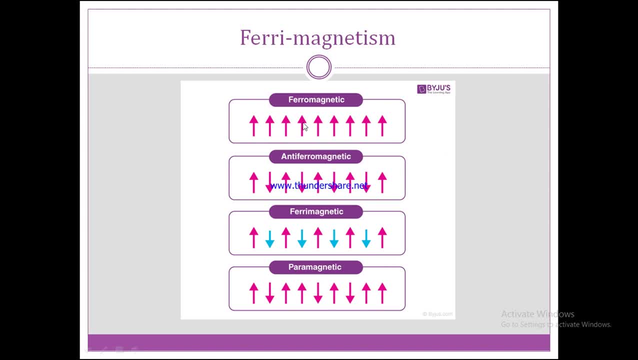 the arrangement of magnetic dipole moments are in a same direction, which are parallel with each other, and the interaction of neighboring dipoles is totally depends upon the parallel structure to each other In anti-ferromagnetic material. 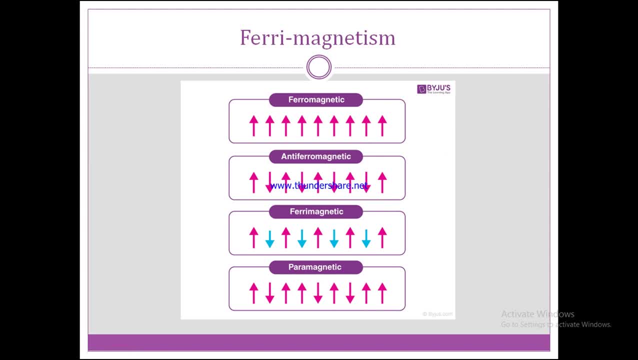 the permanent dipoles are present. the arrangement of anti-ferromagnetic material is such a way that the magnetic dipole moments are opposed to each other and the interaction between neighboring dipoles is the anti-parallel orientation of. 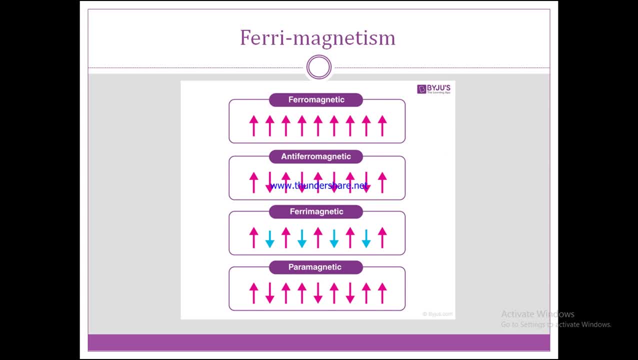 the orientation of equal moments, The last one, that is nothing but the ferromagnetic material. the structure of that ferromagnetic material is shown in this figure, at figure number 3.. The permanent dipole moments are present and the arrangement of dipole moments. 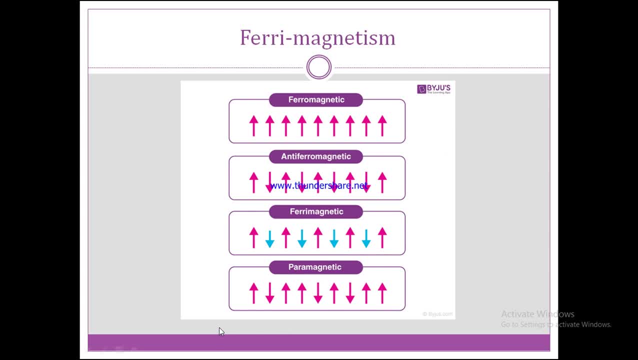 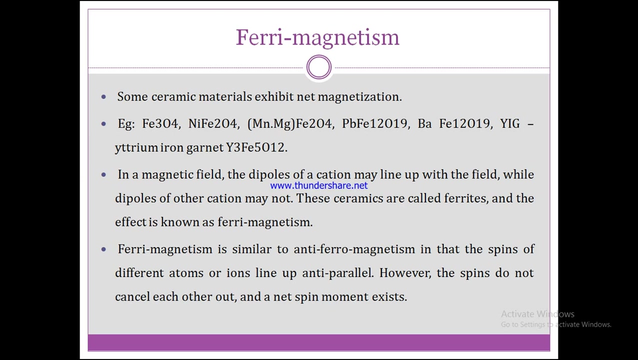 is having the opposite directions, with parallel nature, and the interaction between the neighboring dipoles is nothing but the anti-parallel orientation of unequal moments. The ferromagnetic material, some ceramic materials, exhibit net magnetization, for example. 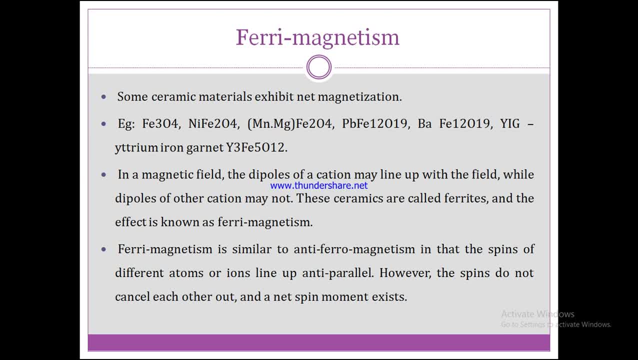 Fe3O4, NiFe2O4, etc. Now, in this type of magnetic field, the dipoles of cation may lines up with the field, while the dipoles of other cation may not. 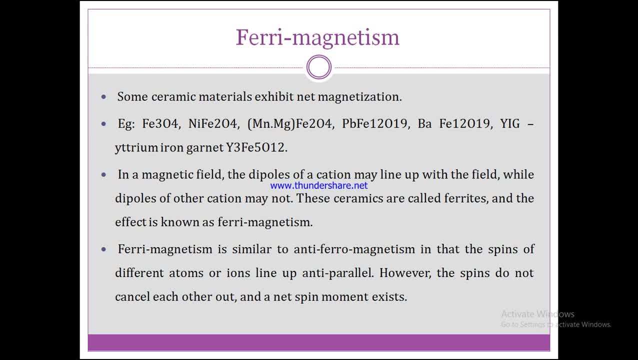 Now these ceramics are called as ferrites and the effect is known as ferrimagnetic. Now, in this type of magnetic field, the dipoles of cation may lines up with the field, while the dipoles of cation 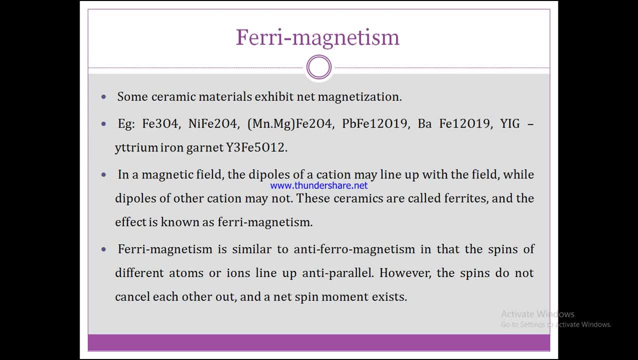 may not. The ferrimagnetism is similar to anti-ferromagnetism in that the spins of different atoms or ions lines up with anti-parallel. However, the spins do not cancel with each other. 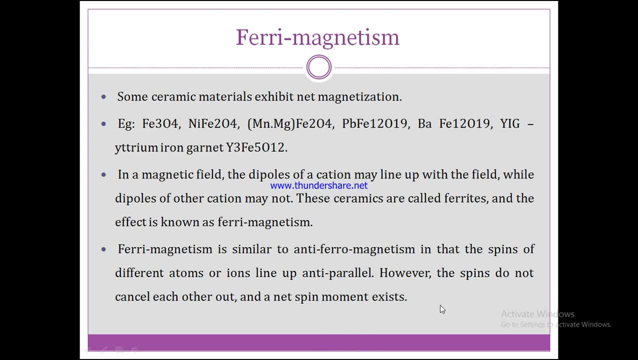 and net spin moment should be exist Now. in a ferrimagnetic material, the dipoles of cation may be lines up with the field as shown in figure, while the dipoles of other cation 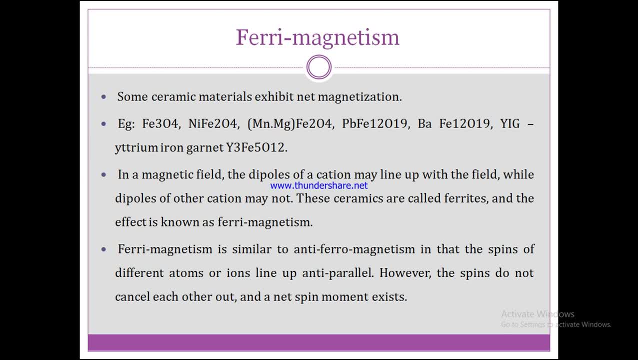 may not. This type of behavior or structure should be called as ferrites, and the effect or the material which effect this type of behavior is known as ferrimagnetism. The ferrimagnetism. 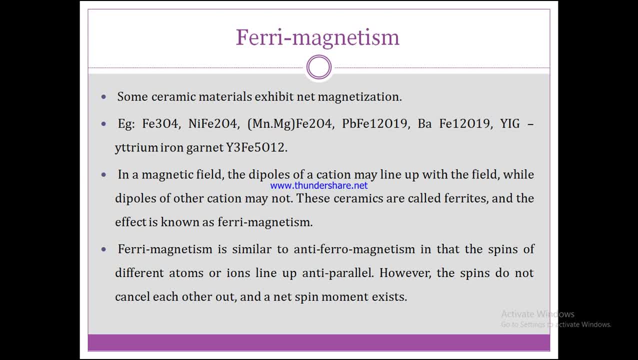 is similar to that of anti-ferromagnetism, which shows that the spins of different atoms or ions lines up with anti-parallel nature. However, the spins do not cancel with each other, and 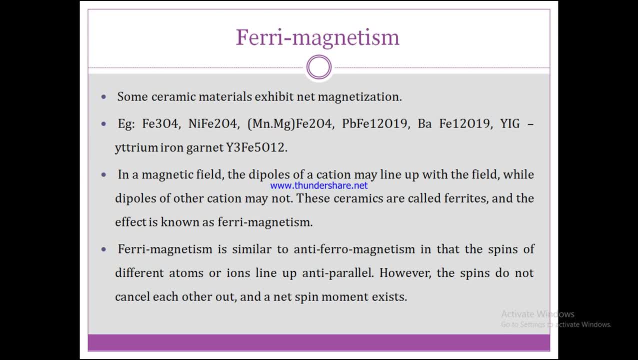 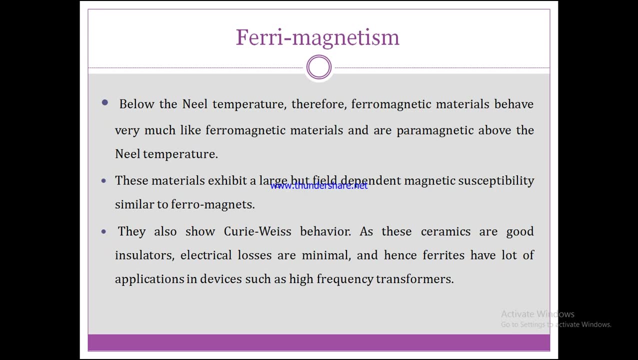 the resultant spin and the resultant spin moment of that particular structure or atom should be exist Now below the mean temperature. the ferrimagnetic materials behave very much like ferrimagnetic materials and are 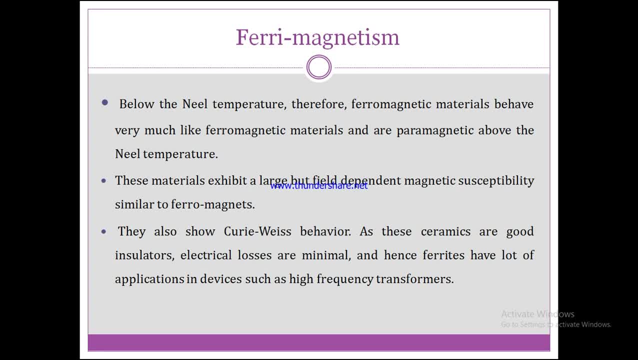 above the mean temperature. As we know, the magnetic material should be depends upon the temperature. below the mean temperature, the ferrimagnetic materials behaves very much like ferrimagnetic material, and above the mean temperature. 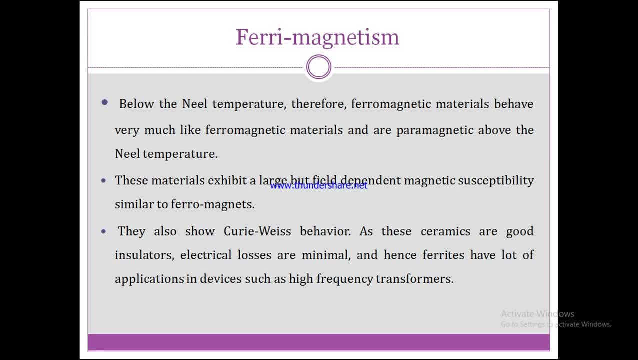 the ferrimagnetic material behaves as an ferrimagnetic material. These materials exhibit a large but field-dependent magnetic susceptibility similar to ferromagnets. The ferrimagnetic materials it should be shows.